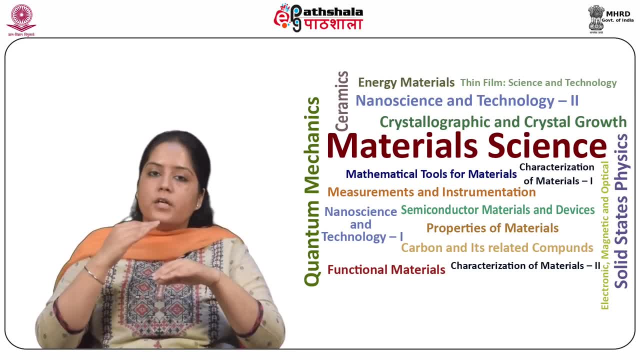 applications, starting from the transformer cores to the data storage devices. In these following sections, we will discuss firstly the basic characteristics of these materials, followed by the fundamental basis of Ferromagnetism. So we are going to talk about the basic characteristics of the Ferromagnet. 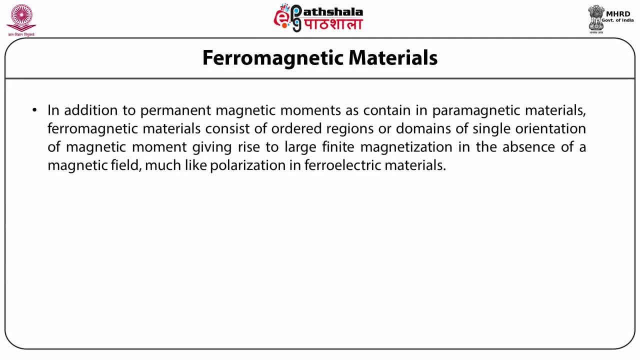 So we are going to talk about the basic characteristics of the Ferromagnet ferromagnetic materials. In addition to permanent magnetic moments as contained in paramagnetic materials, ferromagnetic materials consist of ordered regions or domains of single orientation of magnetic moment giving rise to large finite magnetization. in the absence of a magnetic 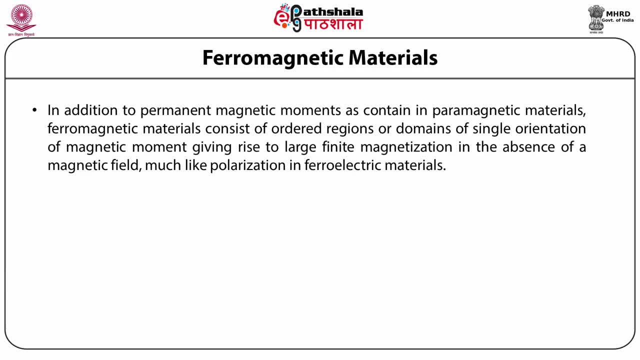 field. This is much like similar to the polarization in ferroelectric materials. This phenomenon is observed below a critical temperature, called as Curie's temperature, above which the material behaves like as a paramagnetic material, As we can see from the figure ie, with no applied. 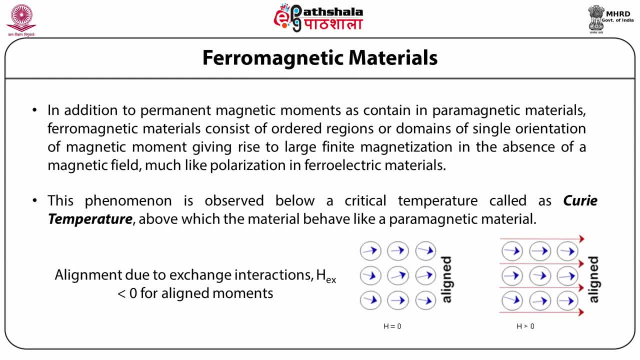 magnetic field, some of the dipoles are aligned, leading to a large magnetic moment. Now, with the application of the applied magnetic field, there are better aligned dipoles, leading to large magnetic moment, large induced moment, and this alignment is due to the exchange interaction for aligned. 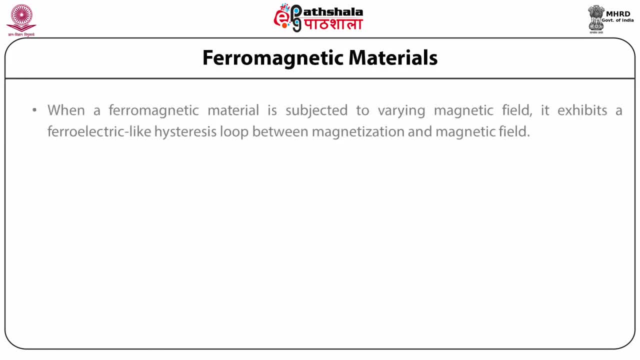 moments When a ferromagnetic material is subjected to varying magnetic field, it exhibits a ferroelectric-like hysteresis loop between the magnetization and magnetic field. A typical ferroelectric loop, which ferromagnetic materials also exhibit, is shown in the figure. 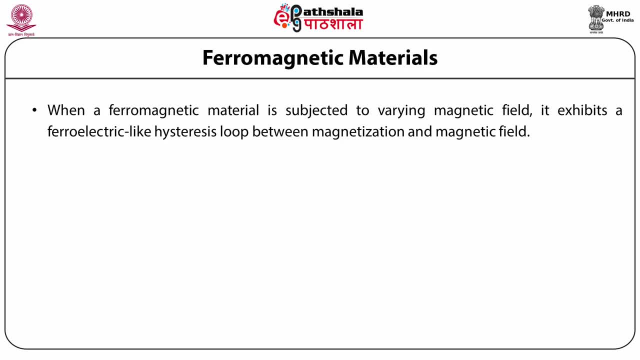 where M is the magnetization and H is the applied magnetic field. Most of the ferromagnetic materials are elemental metals such as iron, nickel, cobalt, etc. However, some oxides, such as chromium oxide, are ferromagnetic oxides. These oxides also tend to be conducting and behave like metals. Now, here there is a. 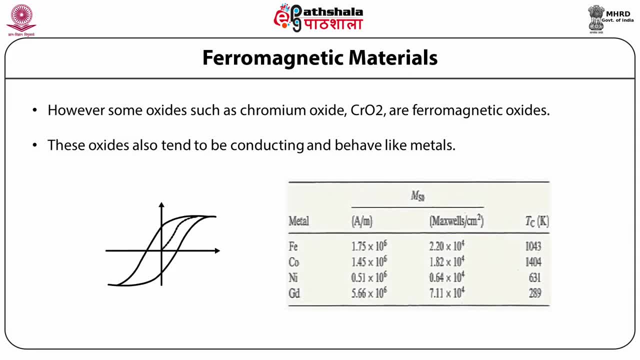 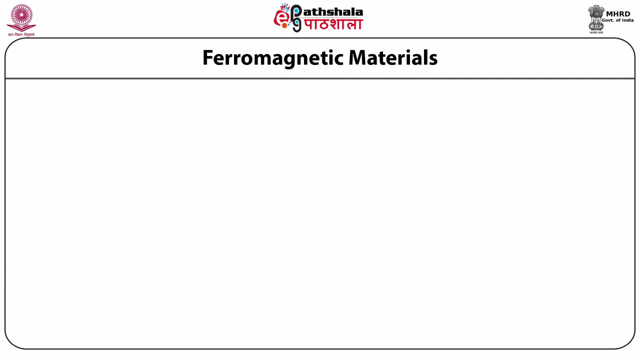 parameter, which is the saturation, magnetization, and it has been tabulated here for all these ferromagnetic metals, Ferromagnetic materials. Now, the ferromagnetic hysteresis loop, as shown in the figure, is due to the domain movement in ferromagnetic materials, The spontaneous 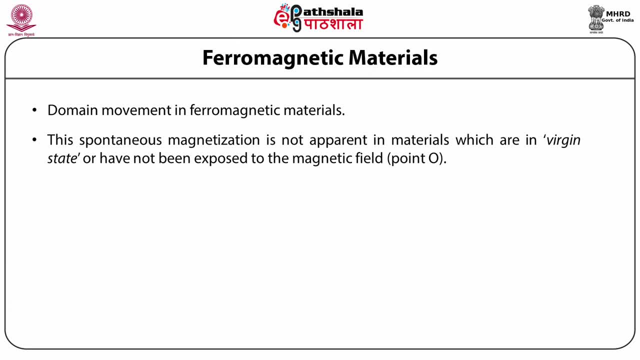 magnetization of the ferromagnetic materials is due to the domain movement in ferromagnetic materials. The spontaneous magnetization is not apparent in the materials which are in virgin state or have not been exposed to the magnetic field, which is represented by the point O in the figure. This is again similar to the case of ferroelectrics, because these materials also contain the domains which are randomly oriented. 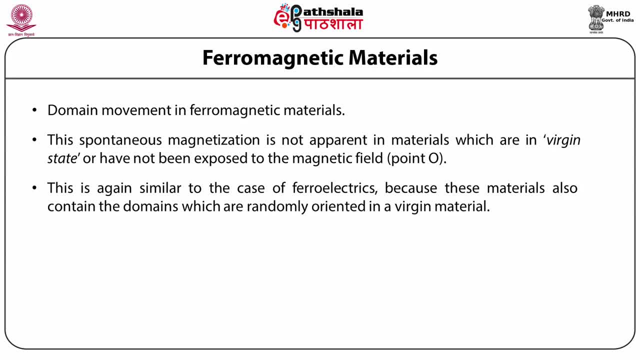 This is again similar to the case of ferroelectrics, because these materials also contain the domains which are randomly oriented in a virgin material. Upon the application of magnetic field, these domains start aligning in the direction of applied magnetic field, which is represented by point B in the figure, and, when completely aligned, give rise to saturation magnetization, ie saturation magnetization. 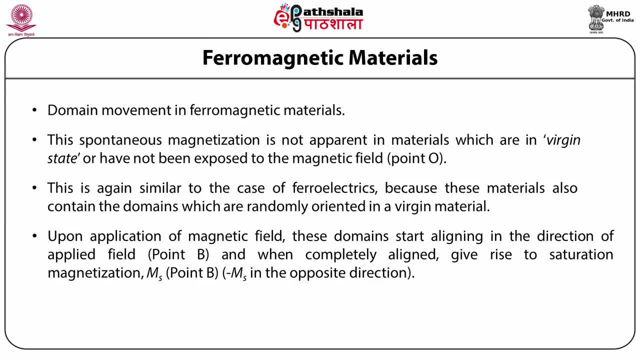 In a spin lot, Bill, and it has a shooting sausages which will be tested to know whether it is irm infused or not. In a spin lot, Bill, and it has a shooting sausages which will be tested to know whether it is irm infused or not. 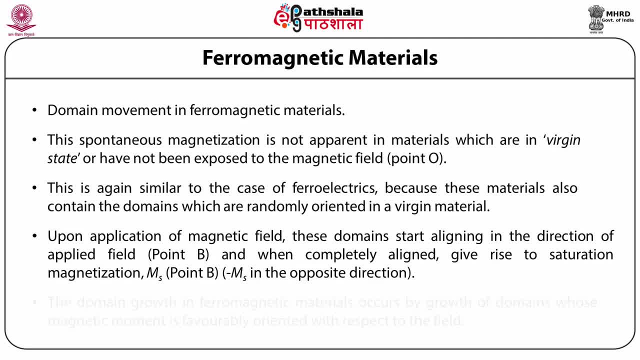 In a spin lot, Bill, and it has a shooting sausages which will be tested to know whether it is irm infused or not. in the opposite direction, The domain growth in ferromagnetic materials occurs by the growth of domains whose magnetic moment is favorably oriented. with respect, 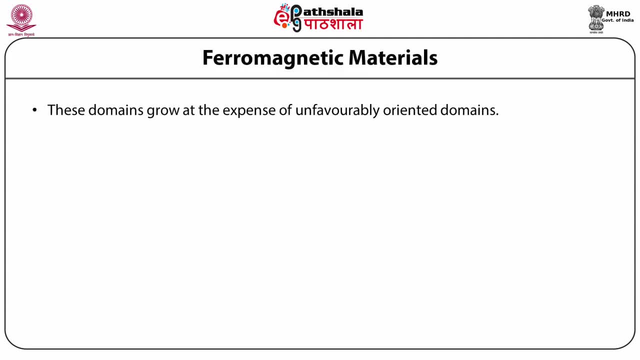 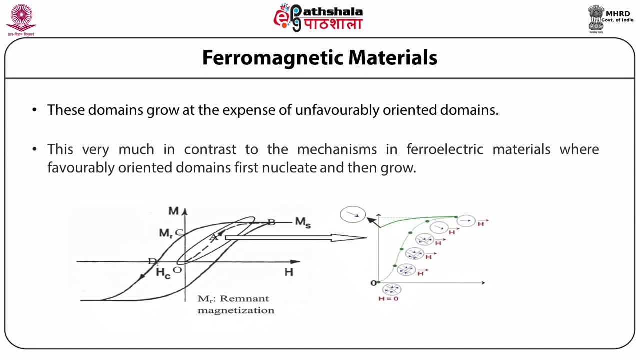 to the field. These domains grow at the expense of which needs increase and decrease, while growing at the expense of unfavourably oriented domains. This very much in contrast to the mechanisms in ferroelectric materials, where favourably oriented domains first nucleate and then grow When the field 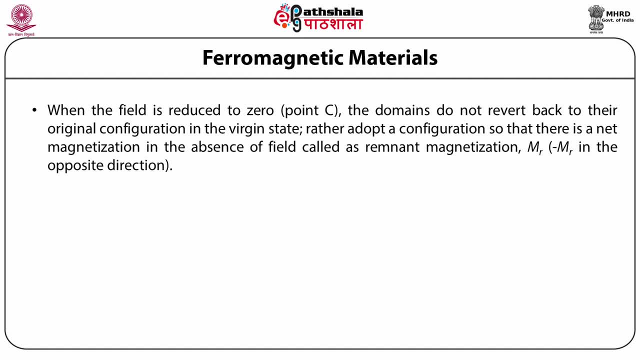 is reduced to 0, which is represented by point C, the domains do not revert back to their original configuration in the virgin state. Rather, they adopt a configuration so that there is a net magnetisation in the absence of field, called as remnant magnetisation, which 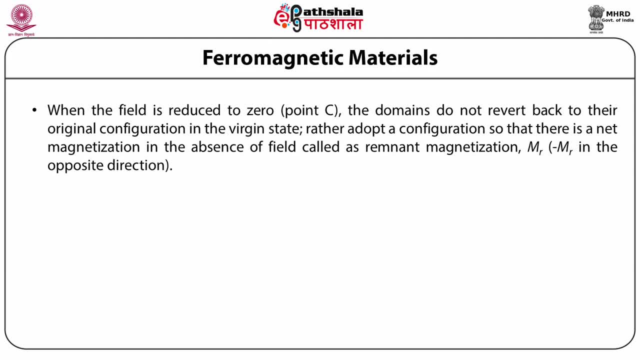 is represented by mR in the graph and minus mr in the opposite direction. To bring the magnetization of the material back to zero, one needs to apply an extra field in the opposite direction, which is called as coercive field, and it is represented by minus hc and plus hc. 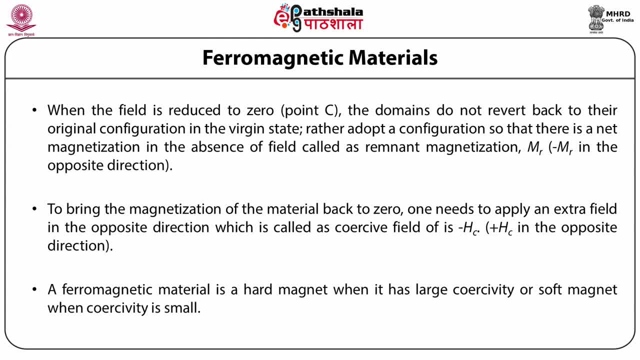 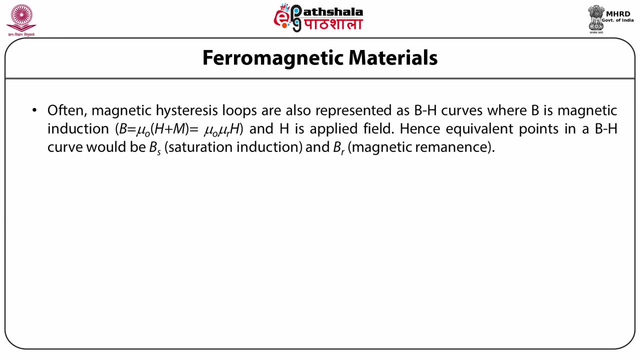 in the opposite direction. A ferromagnetic material is a hard magnet when it has large coercivity or soft magnet when coercivity is small. Often magnetic hysteresis loops are also represented as bh curves. where b is magnetic induction, b is equal to mu naught. 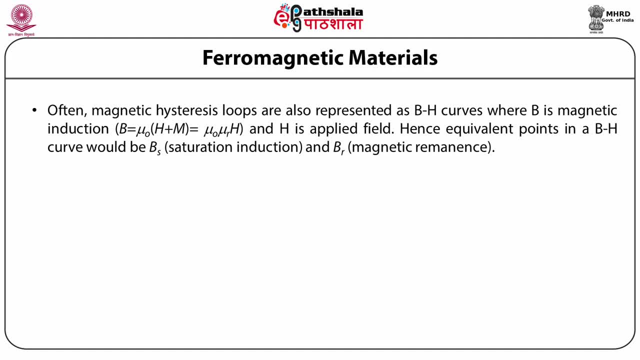 h plus m, or it is equal to mu, naught, mu r, h, where h is the applied magnetic field. Hence the equivalent points in a bh curve would be bs, the saturation induction, and br, the magnetic remnants, As evident from the figure that this circled part has been zoomed. 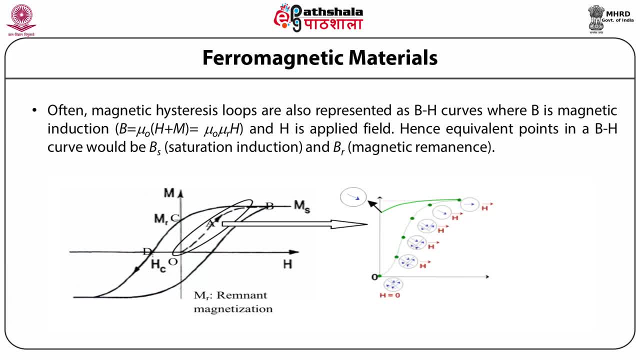 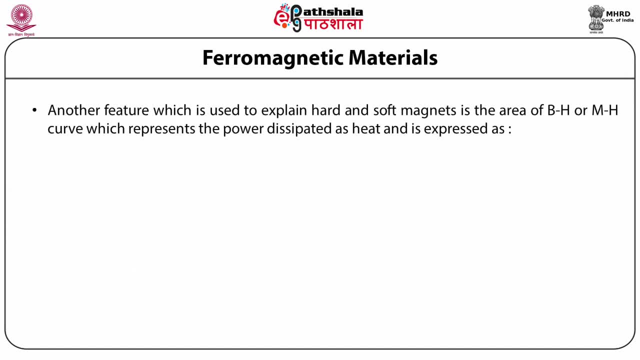 out. Another feature which is used to explain hard and soft magnets is the area of bh curve, which represents the power dissipated as heat, and it can be expressed as m導 h and the heat dissipated as denser. The flux of heat is the area of the magnet, which is the contact area of the magnet, and 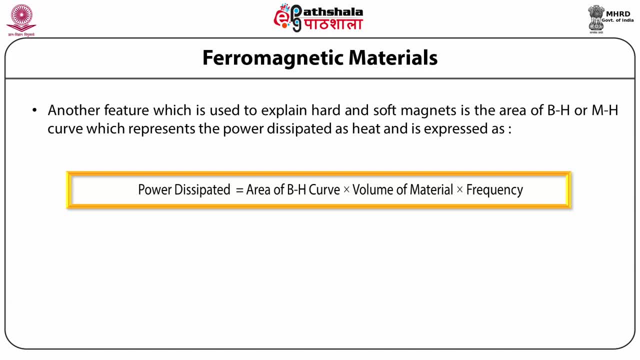 the magnetic magnet. The force of current is the heat, which is also the force of the magnetic field, and the force of the magnet is the surface. The force of the magnetic field is the force of the magnet Power dissipated is equal to the area of pH curve multiplied by the volume of the material. 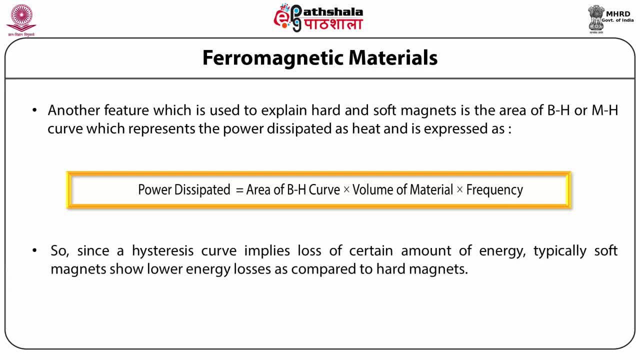 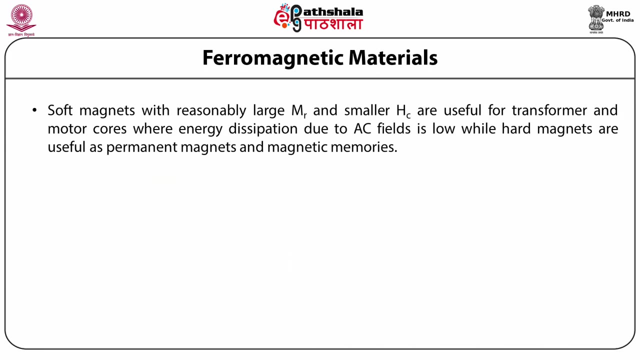 multiplied by the frequency. So since a hysteresis curve implies loss of certain amount of energy, typically soft magnets show lower energy losses as compared to hard magnets. Soft magnets with reasonably large MR and smaller HC and smaller HC are useful for transformer. 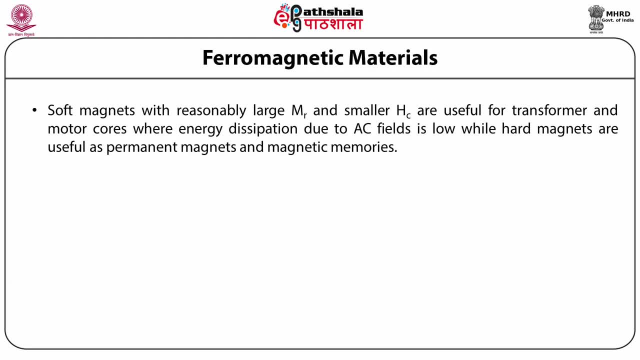 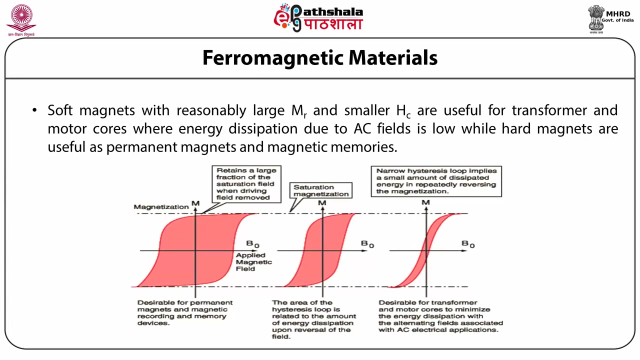 and motor cores where energy dissipation due to AC is not possible. So soft magnets with reasonably large MR and smaller HC are useful, for AC fields is low, while hard magnets are useful as permanent magnets and magnetic memories, As it is clear from the figure that the pH curve which is represented by the first figure, 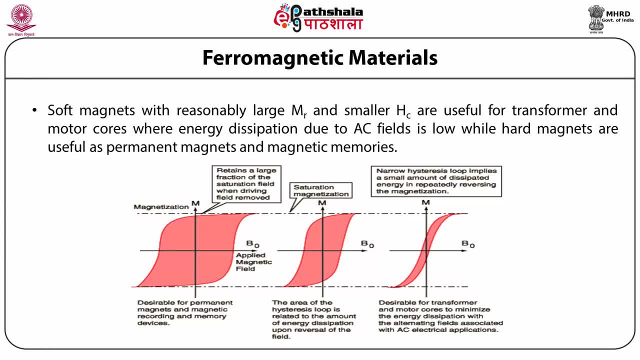 where it has a large M and HC desirable for permanent magnets and magnetic recording and memory devices. It retains a large fraction of saturation field when driving field is removed. The second graph shows that the area of the hysteresis loop is smaller than that of the previous graph and it is related to the amount of energy dissipation. 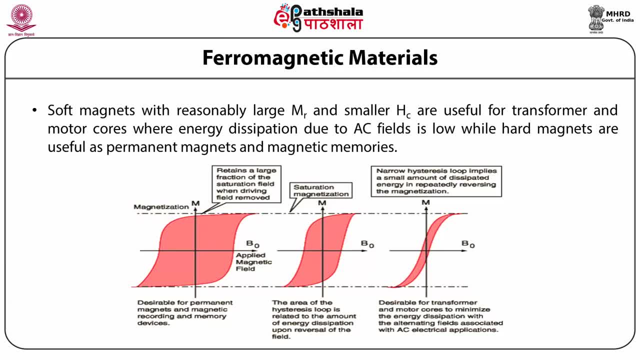 upon the reversal of the field. The third graph is the narrow hysteresis loop, that is, having smaller energy dissipation. It desirable for transformer and motor cores to minimize the energy dissipation with the alternating fields associated with ac electrical applications. pity Butranti, This is above the это examples with AC electrical applications. 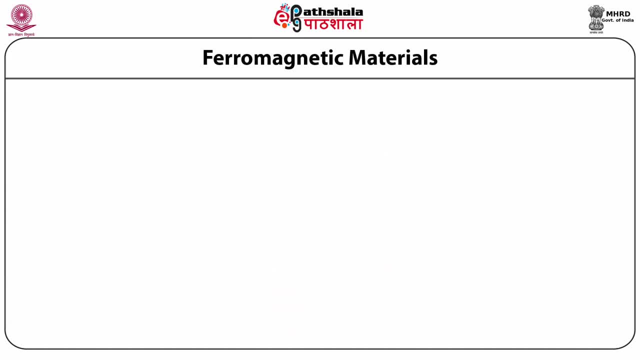 This figure shows that what is going on is separate energy dissipation: tube current, CO2. The figure shows the formation of domains in a ferromagnetic material. As we can see from the figure that the flux lines on the surface of a magnet in mono domain 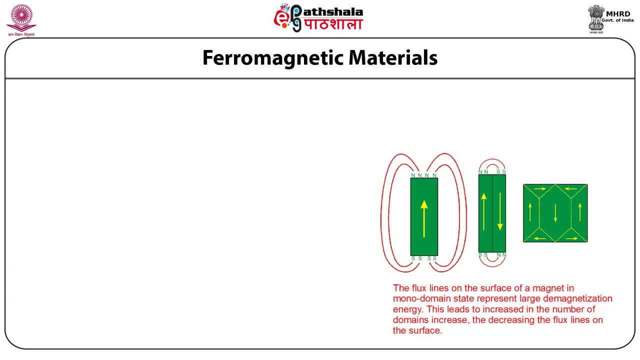 state represents large demagnetization energy. This leads to increase in the number of domain and the decreasing the flux lines on the surface. Again, the formation of domains and their size in these materials is basically due to balance between various kinds of energies associated. First is the exchange energy. 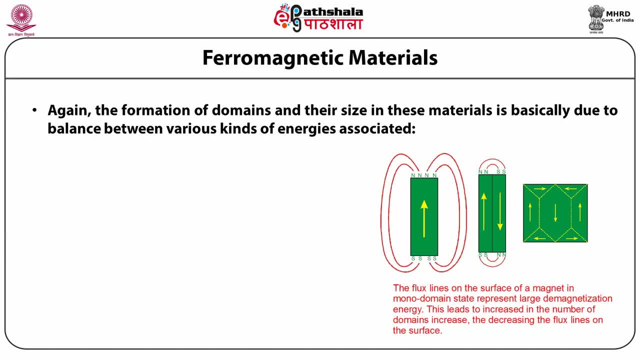 Which is the energy exchange energy Which makes the magnetic moments align in one direction without violating the Pauli's exclusion principle. Second is the magnetostatic energy in response to the flux lines at the surface of the material in the mono domain state, Which increases as alignment increases. 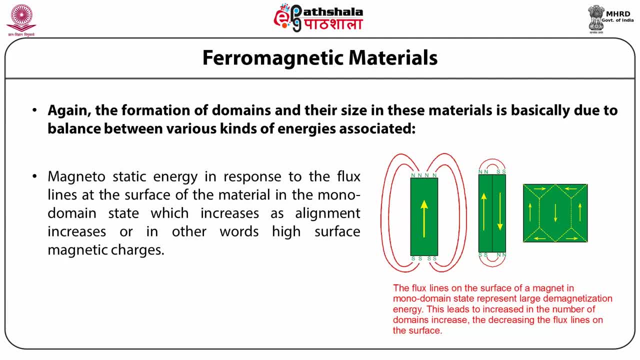 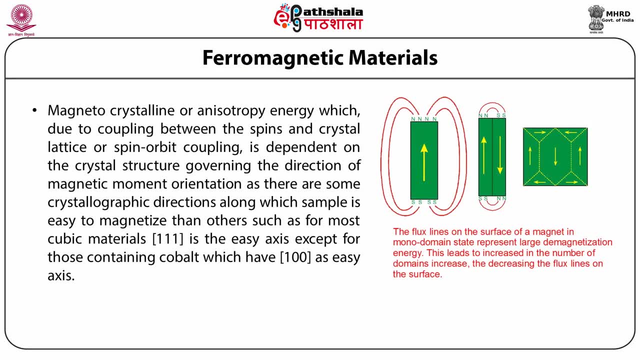 Or in other words high surface magnetic charges. Third is the magnetocrystalline or anisotropy energy Which is due to the coupling between the spins and the crystal lattice, or spin orbit coupling. It is dependent on the crystal structure governing the direction of magnetic moment orientation. 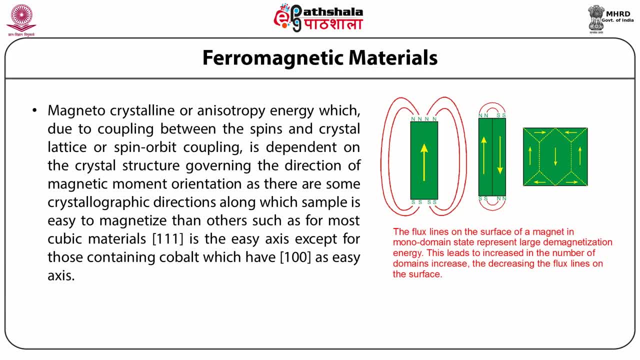 And the después is due to further unoct啵 that in the period at which the writers made a particular analogy about magnetos, with some sparkle on the surface and some hertz ghost. here, The example we're going to see next a one is the magnetambling gesture along which 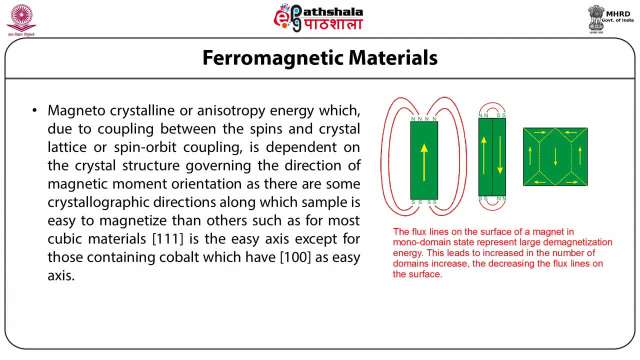 sample is easy to magnetize than others, such as for most cubic materials, Such asCTB is the easy axis, except for those containing cobalt, Which have 1, 0,0 as the easy axis. The normal cognitiveness of other magnets is decrease because the magnetos are hard to. 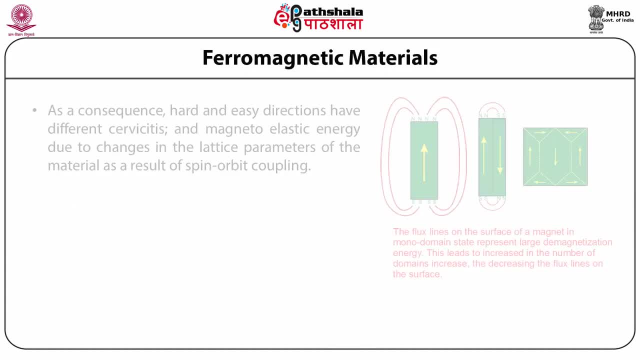 climbed, which is establishment fantasy. now here are someبs. because first we have magnetตadi twink than alveoli or the matrix at x, prime starत we consider as a cobalt number within the cobalt number. So if firstt dr k Be just like and first slow down symbol by saying thenacon td between 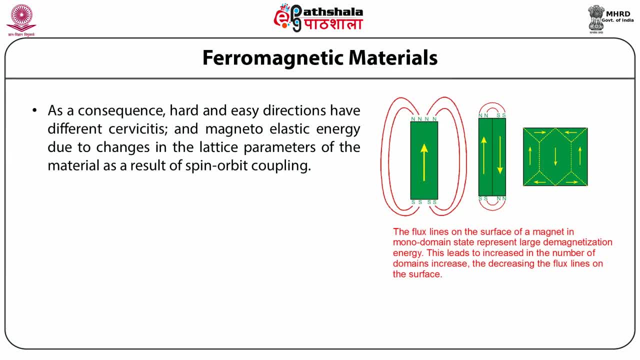 As a consequence, hard and easy directions have different coercivities. Lastly, is the magnetoelastic energy, which is due to the changes in the lattice parameters of the material as a result of spin-orbit coupling. The phenomenon is called as magnetostriction and it is quite useful from application point of view. 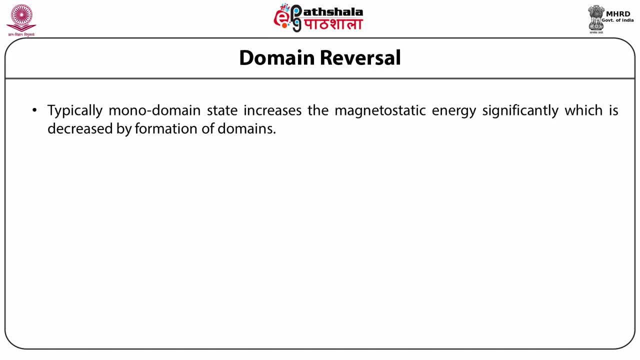 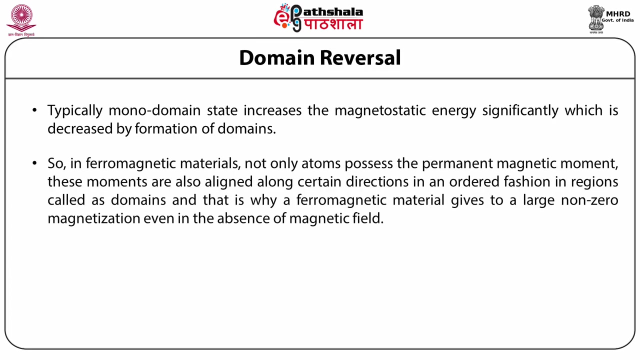 Typically monodomain state increases the magnetostatic energy significantly, which is decreased by the formation of domains, Although existence of multidomain state also requires a surface. In the case of surface energy, the phenomenon is energetically stable. In ferromagnetic materials, not only atoms possess the permanent magnetic moment. 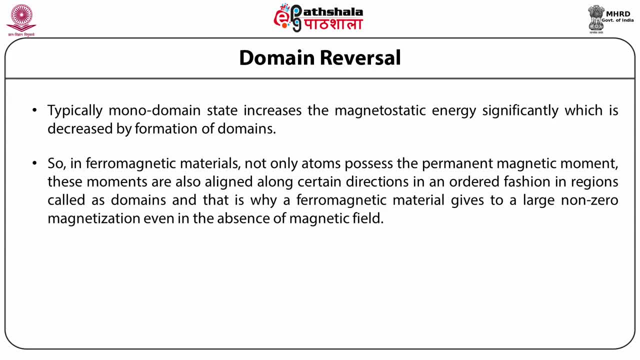 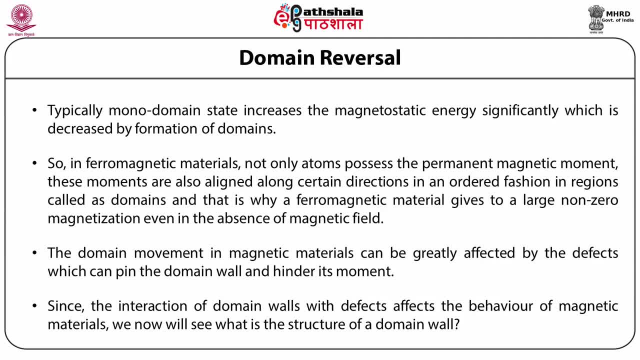 That is why ferromagnetic material gives to a large, non-zero magnetization, even in the absence of magnetic field moments or magnetic materials. we will now study how does. a domain wall is formed, which is leading to the domain reversal, and this domain reversal is leading to the hysteresis loop. a domain wall is often called as the block wall. 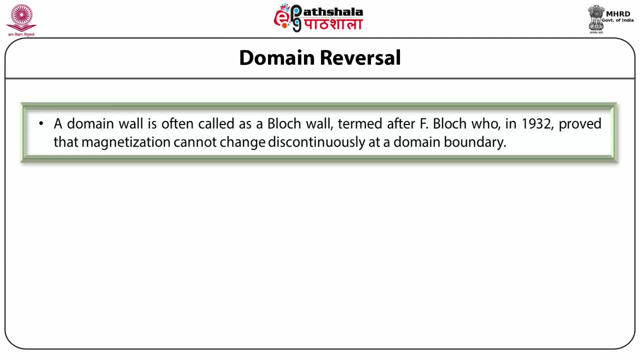 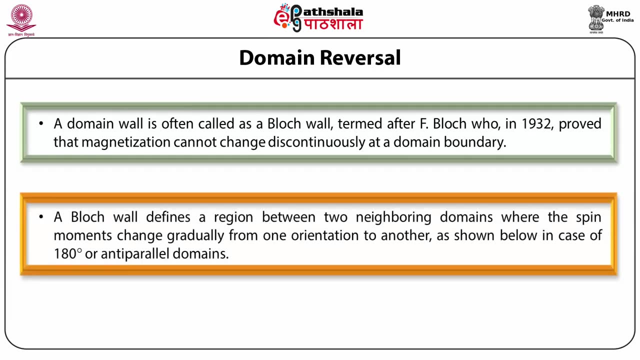 which is termed after F law in 1932 proved that the magnetization cannot change discontinuously at a domain boundary. a block wall defines a region between two neighboring domains where the spin moments change gradually from one orientation to another, as shown in the figure in case of 180 degree or anti-parallel domains. block 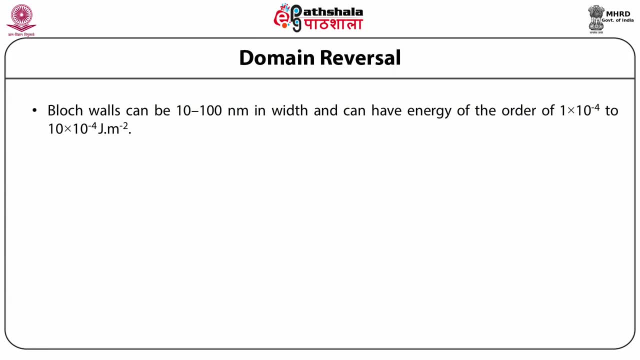 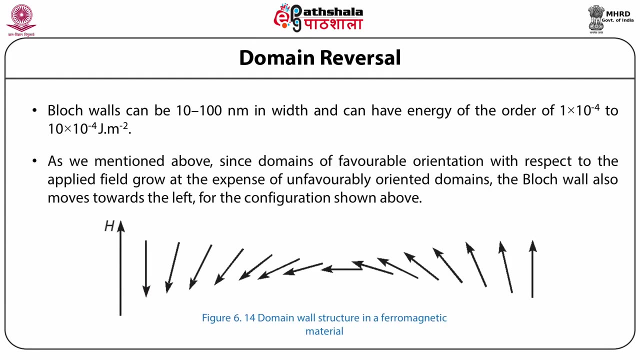 walls can be 10 to 100 nanometer in width and can have an energy of the order of 10 to the power minus 4 to 10 multiplied by 10 to the power minus 4 joules per meter square, as we have mentioned above. since domains of 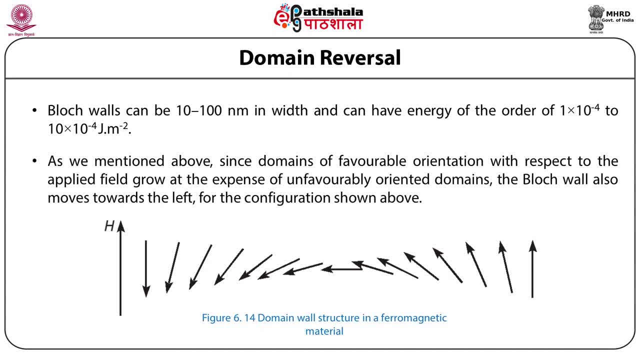 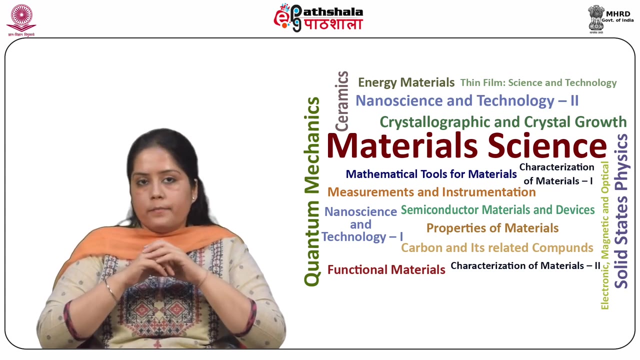 favorable orientations can change depending on the orientation of the region with respect to the applied field, grow at the expense of unfavorably oriented domains. the block wall also moves towards the left, as shown in the figure. microscopic reasons of ferromagnetism: derivation of the Curie's. 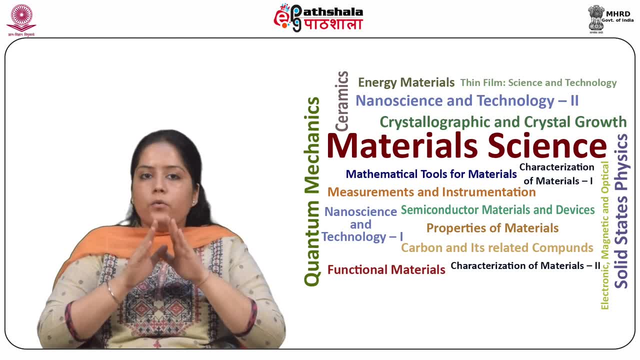 law assumed that. the law assumed that the law assumed that the localized atomic magnetic moments do not interact with each other at all. they are localized atomic magnetic moments do not interact with each other at all. they are just reoriented by the applied magnetic field. V's explained the observed Curie. 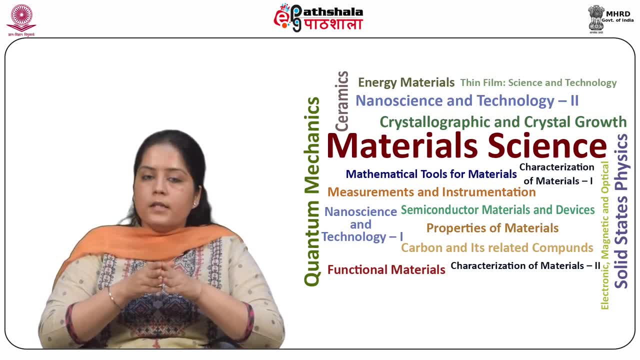 V's behavior by postulating the existence of an internal interaction between the just reented the expected state until these moments depended on the local deity. the leder He farkt matter. movement of the sla희가. the leder He farkt matter. movement of the slaaska. 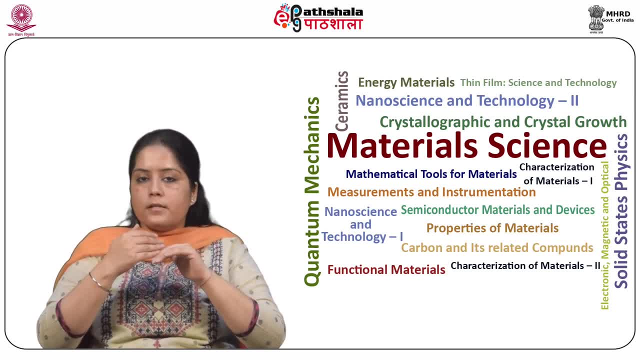 the localized moment, mystical study or molecular field. he did not speculate as to the origin of this molecular field beyond suggesting that it is a mutual interaction between the electrons which tends to align the dipole moments parallel to the Sarac deutlichii to each other. We can't really criticize Wyss for this. Remember that the electron 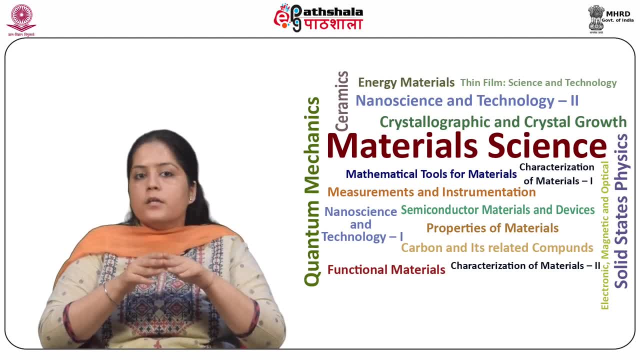 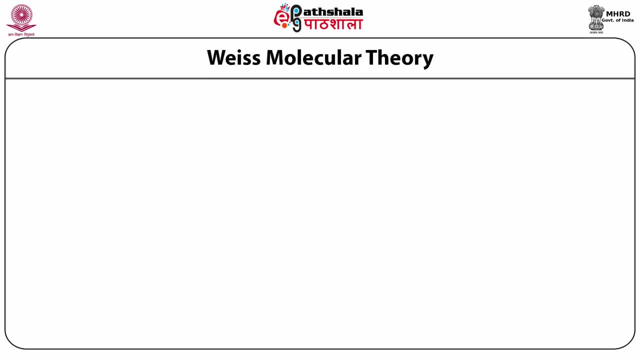 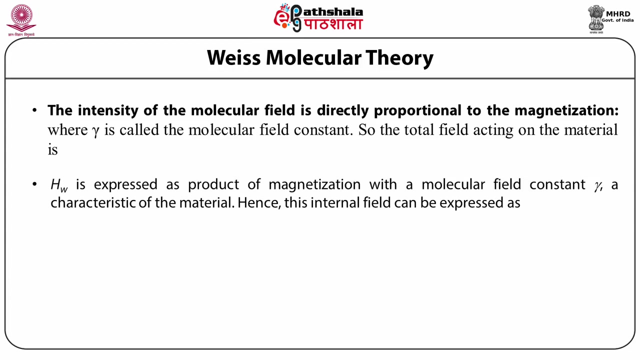 had been discovered only 10 years earlier and the quantum mechanics hadn't been invented yet. The Wyss molecular theory, The intensity of the molecular field, that is Hw, is directly proportional to the magnetization, and hence this Hw is expressed as the product of magnetization. 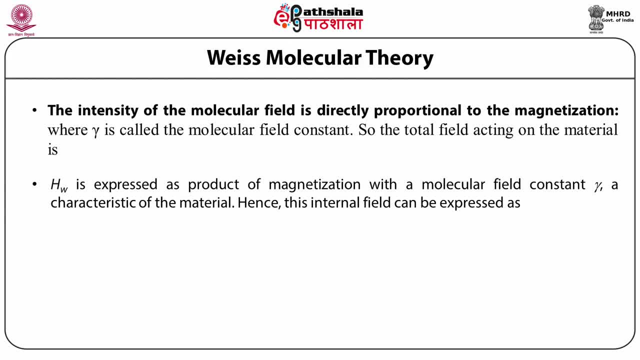 with a molecular field, constant gamma, which is a characteristic of the magnetic field. Hence the internal field, or we can say the total field which is acting on the material, is the summation of H plus Hw. Now we can put the value of Hw, then the H total will. 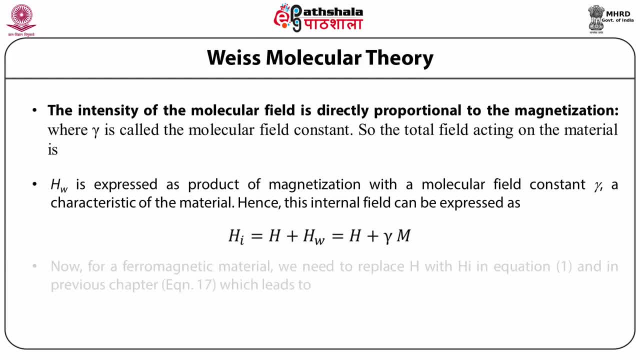 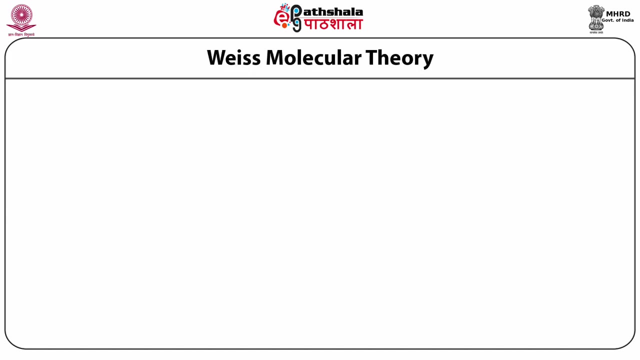 become H plus gamma m. Now for a ferromagnetic material we need to replace H with gamma m, So Hw is equal to H total, and hence this susceptibility, which is equal to m by H, or it is equal to C by T. Here we will put the value of H as H total, Hence m by H plus. 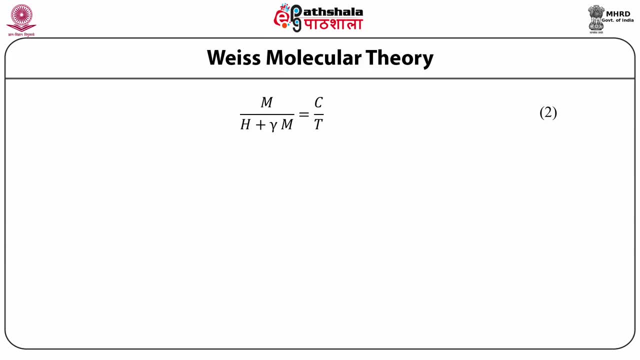 gamma m will be equal to C by T. This implies that m is equal to C multiplied by H, divided by Hw, T minus gamma C. So finally we will get the ratio of m by H is equal to C by T minus theta, where theta is equal to gamma C and it has a unit of temperature and is called 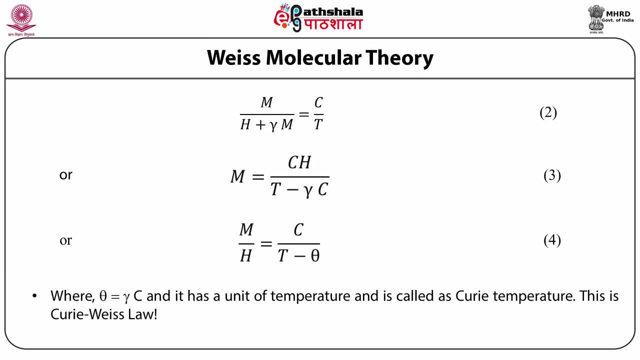 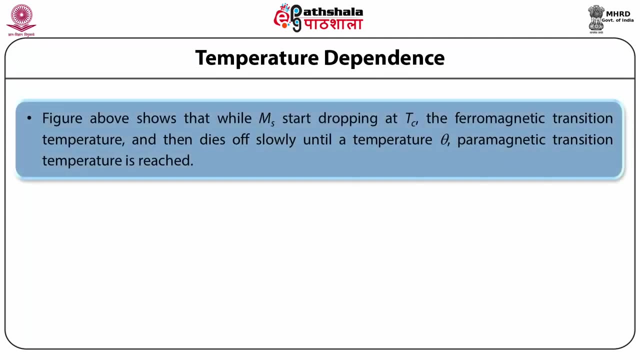 as the Curie temperature. This is also called as the Curie-Wyss law, The temperature dependence of magnetization or susceptibility. The figure shows that while ms starts dropping at T equal to Tc, the ferromagnetic transition temperature, and then it dies off slowly until a temperature theta, which is the paramagnetic transition. 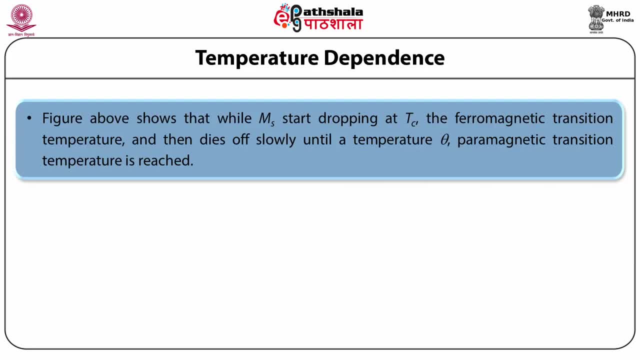 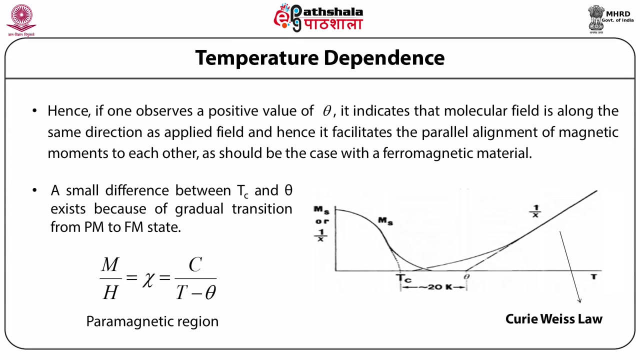 temperature. Now there is a divergence in susceptibility. inverse at T is equal to theta in the paramagnetic region, which is a signature of a phase transition to a magnetically ordered phase with spontaneous magnetization. Hence if one observes a positive value of theta, it indicates that molecular field. 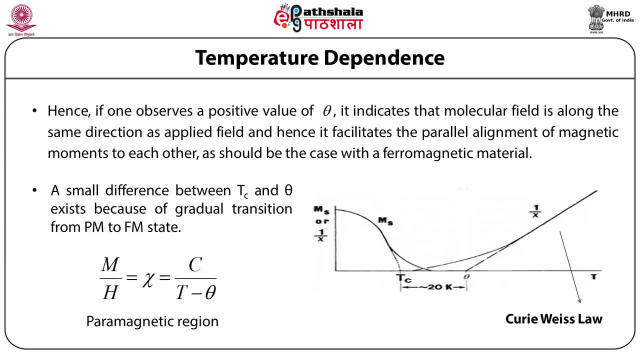 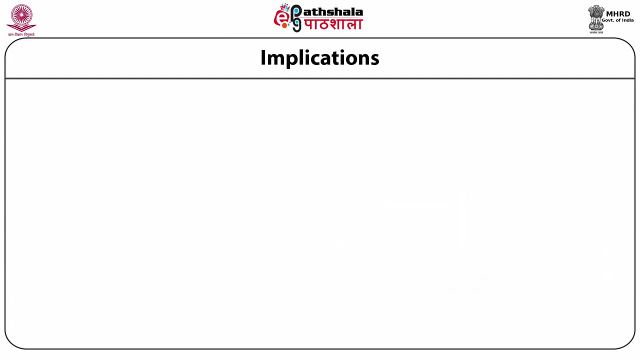 is along the same direction as applied field, and hence it facilitates the parallel alignment of magnetic moments to each other, as should be the case with a Ferromagnetic material material. So, students, let us discuss. what are the implications of this Curie-Weiss law. 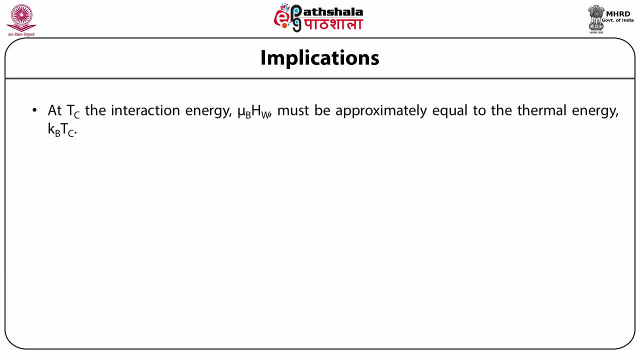 At Tc, the interaction energy, that is mu B, HW must be approximately equal to the thermal energy which is KB Tc. So for a material with a Curie temperature of around 1000 Kelvin the HW will be equal to 10 to the power 3 OSTED, and this is a very large field. 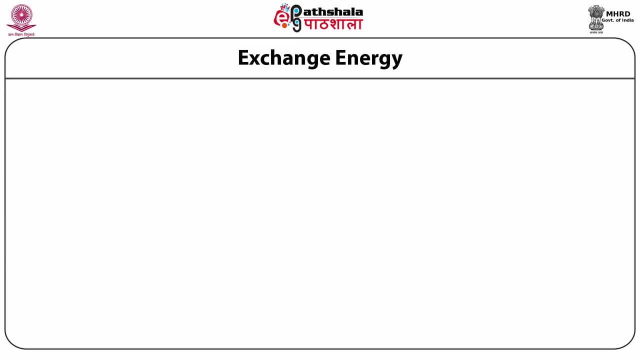 Exchange energy Students. let me mention here that exchange energy is a very large field. So exchange energy is a very large field. The origin of Weiss molecular field is the exchange interaction as a combined consequence of the Pauli's exclusion principle, as well as the Coulombic interactions between the electrons. 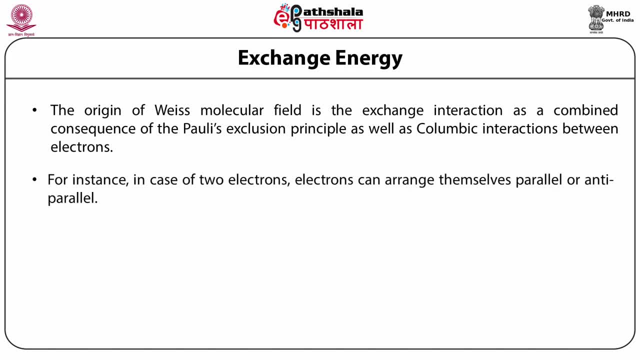 For instance, in case of two electrons, they can arrange themselves parallel or antiparallel. If parallel, they can arrange themselves in a parallel or antiparallel way. If parallel, Pauli's exclusion principle requires them to remain far apart, and if antiparallel, 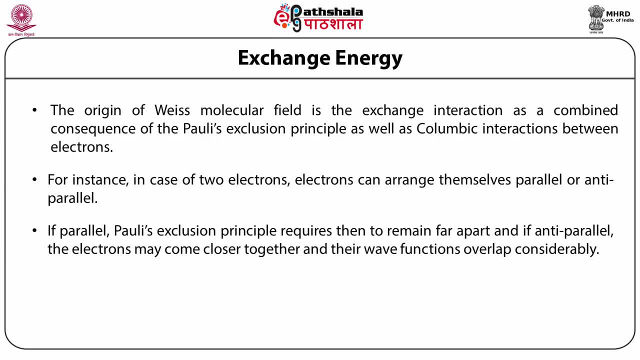 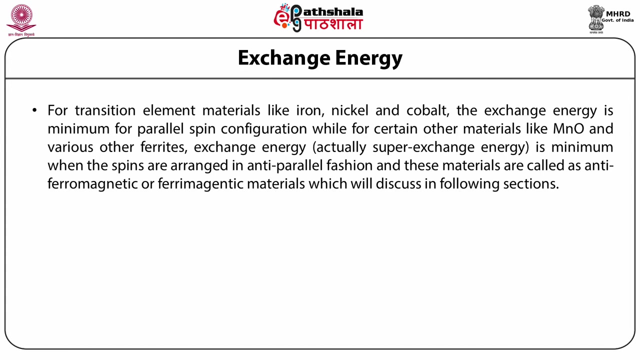 the electrons may come closer together and their wave functions overlap considerably. Hence the electrostatic energy of the electron system is governed by the relative orientation of the spins with respect to each other either, and the difference in the energy is a manifestation of the exchange energy For transition element materials like iron, nickel and cobalt. 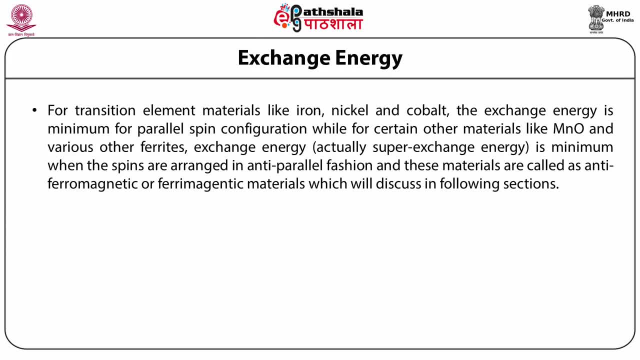 the exchange energy is minimum for parallel spin configuration, while for certain other materials, like MnM7, yet b nest intermediate cellENE, the exchange ninguém kann überwysical. The exchange energy is minimum when the spins are arranged in antiparallel fashion and 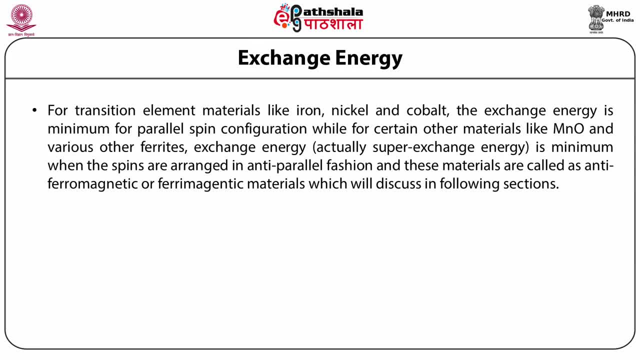 these materials are called as anti-ferromagnetic or ferrimagnetic material. The exchange interaction is a short-range interaction and hence the similarity between the Conservative CAP possibilities per different spin containers is quite significant. Also, the uninterrupted interactions are the most oil- scars. lead summation: MotorР. 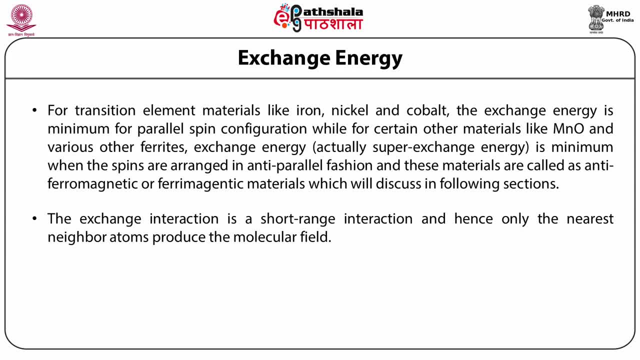 XXV-2 inter-variation. The faster tetrahedron interacts with the right frontier, the faster the silicon molto market space, sinisterly Moving through an anterior engine phase. the moreз neighbor atoms produce the molecular field, The magnitude of exchange or molecular field. 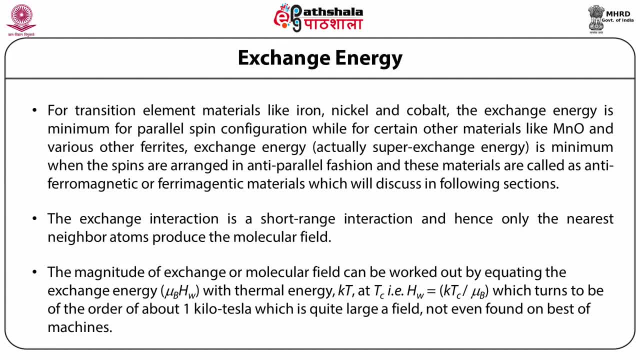 can be worked out by equating the exchange energy, that is, mu B, HW, with thermal energy, kT at Tc ie HW is equal to kTc by mu B, which turns out to be the order of 1 kT. and as we 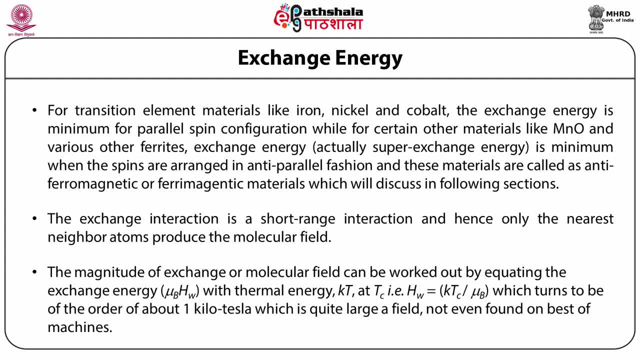 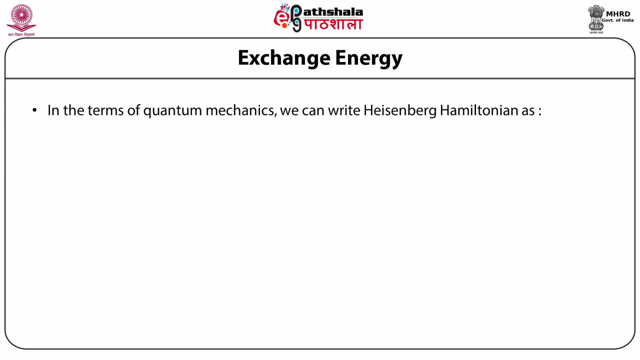 have previously mentioned that this is a very large field In terms of quantum mechanics. we can write Heisenberg Hamiltonian as h exchange is equal to minus summation over i, j, j exchange, S, i multiplied by S, j, where j exchange is equal to the integral over phi. a star as a. 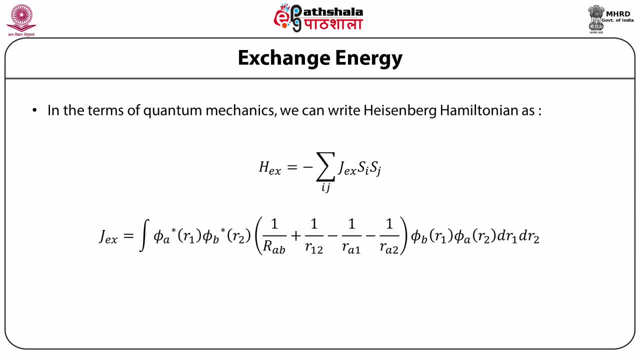 function of r1.. phi b star as a function of r2.. This whole multiplied by bracket 1, by r a, b plus 1, by r1, 2 minus 1, by r a, 1 minus 1, by r a, 2, bracket close, multiplied by phi b, r1, phi a, r2, d, r1 d, r2.. j is being positive. 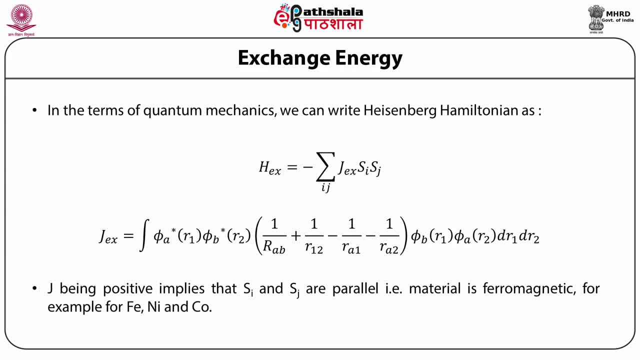 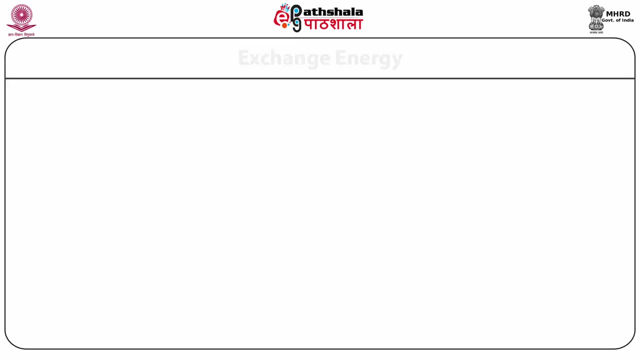 implies that S i and S j are parallel. ie material is ferromagnetic, For example, as we can see from the figure, for iron and nickel and cobalt. On the other hand, a negative value of j implies anti-ferromagnetic ordering, as we can see from the figure, the materials like chromium. 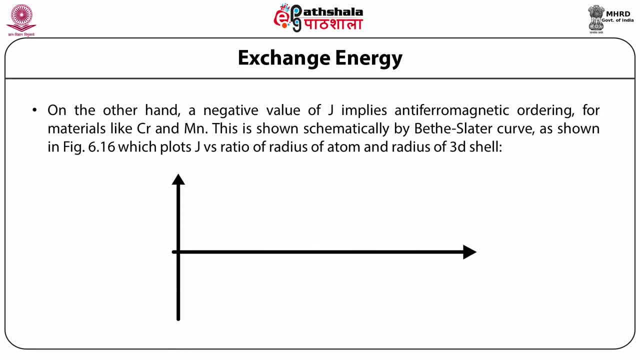 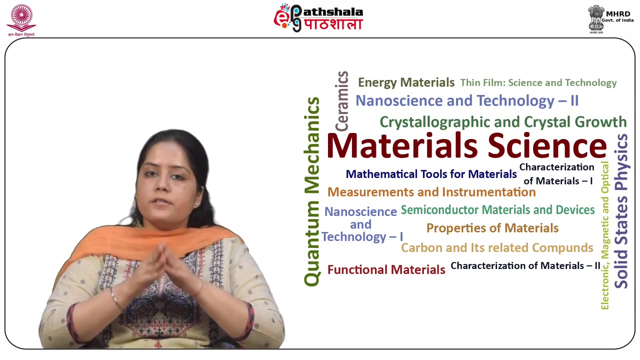 and manganese. The figure is a Bethe-Slatter curve which shows the plot between j versus the ratio of the radius of atom and the radius of 3D shell. So, students, let us summarize what we have learnt in this module. First, the ferromagnetism.